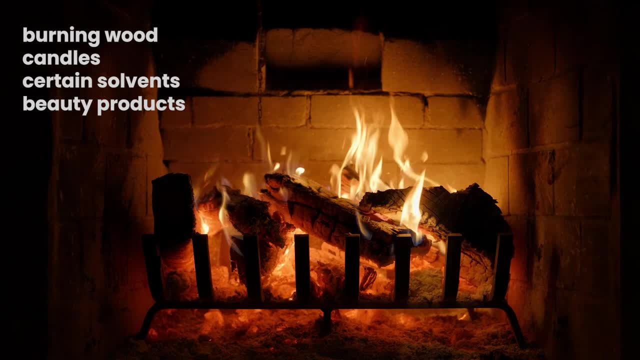 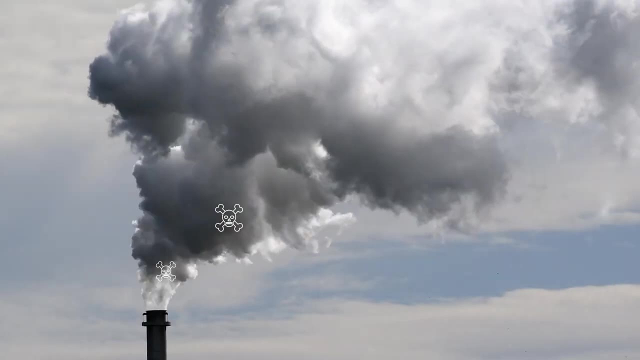 Indoors. our activities, such as burning wood candles and using certain solvents and beauty products, can increase how much we are exposed to particulate matter pollution. Why does it matter? Research tells us that there are no safe levels of air pollution and any exposure to it can be harmful to health, shortening our lives and reducing healthy life years. 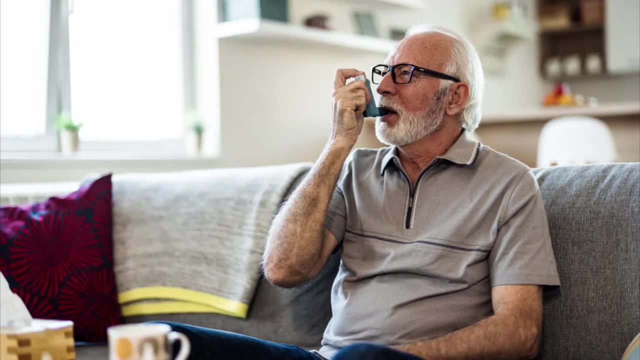 Air pollution affects everyone, but some people are more vulnerable to its effects than others. This includes older people and specifically those with a long-term health condition such as a lung or heart problem, including chronic obstructive pulmonary disease, asthma or coronary heart disease. 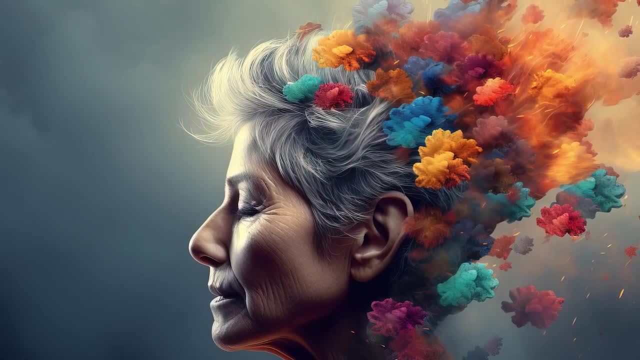 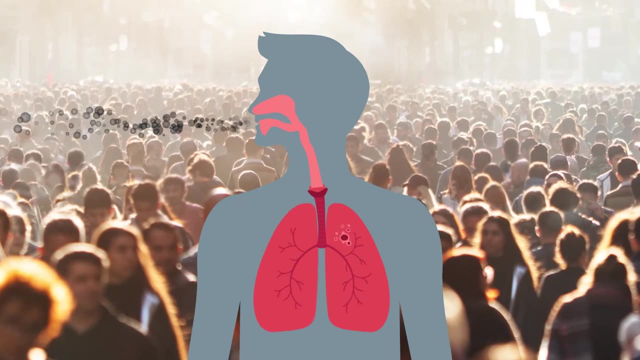 New research also suggests air pollution can lead to memory decline and dementia. When we breathe in polluted air, the particles can get stuck in our lungs or, in some cases, if they are small enough, they pass through the lungs and into the bloodstream. 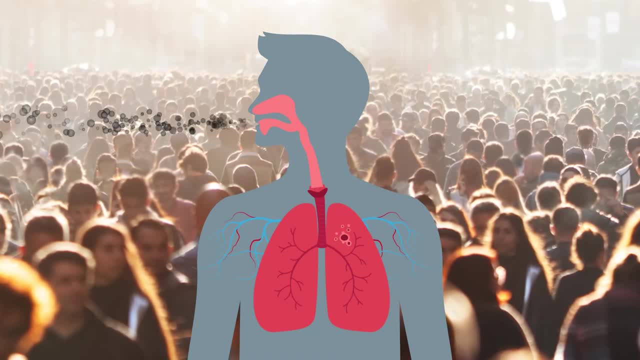 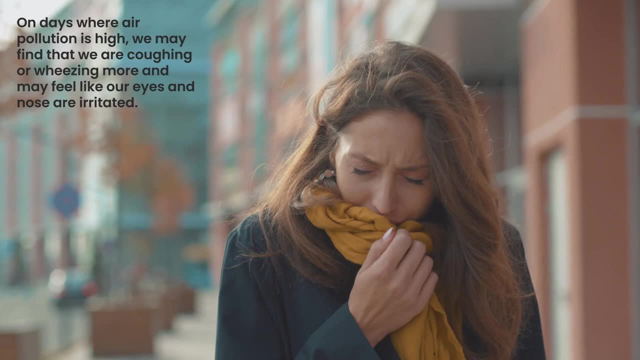 Air pollution can irritate our airways and irritate any lung illness that we already experience. On days where air pollution is high, we may find that we are coughing or wheezing more and may feel like our eyes and nose are irritated. 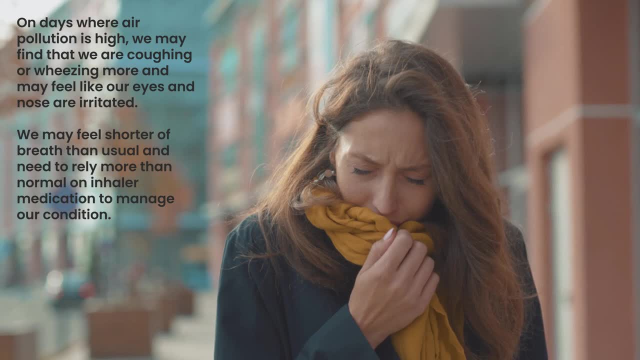 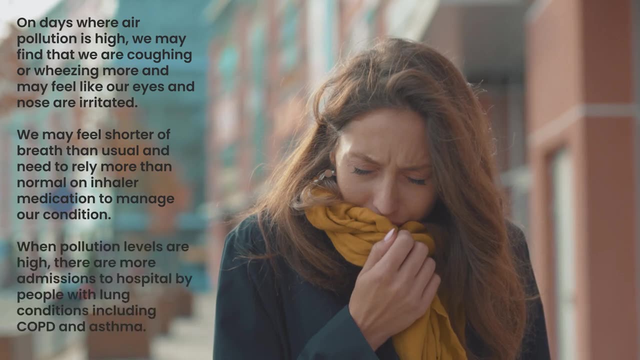 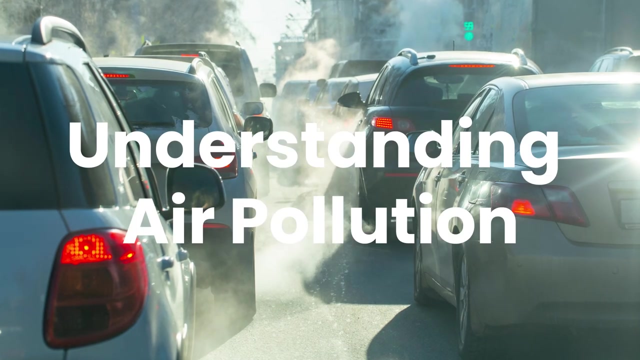 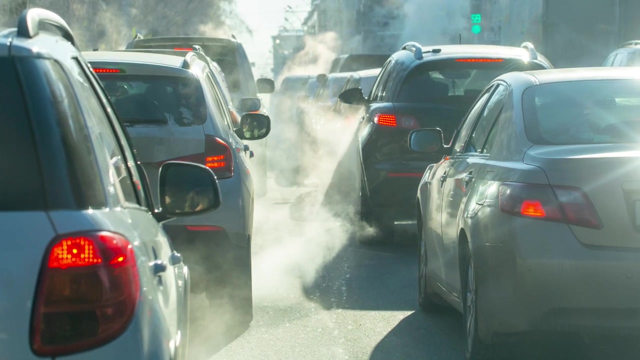 We may feel shorter of breath than usual and need to rely more than normal on inhaler medication to manage our condition. When pollution levels are high, there are more admissions to hospital by people with lung conditions, including asthma. Understanding air pollution, We often think of air pollution being something that affects us when we are outdoors from traffic and industry, yet many pollutants are also found in our indoor environment, where we spend approximately 90% of our time. 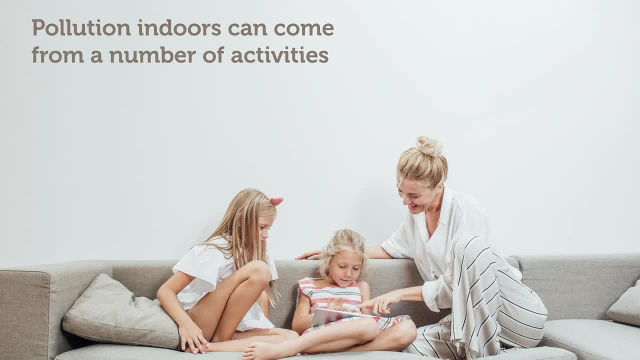 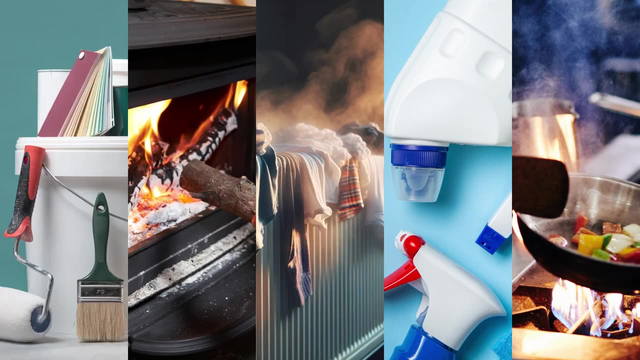 Pollution indoors can come from a number of activities. Pollution indoors can come from a number of activities, Such as cooking, cleaning, drying clothes, burning wood or candles, and using certain personal care or decorating products. Breathing polluted air indoors can make symptoms of heart and lung conditions, as well as allergies, worse. 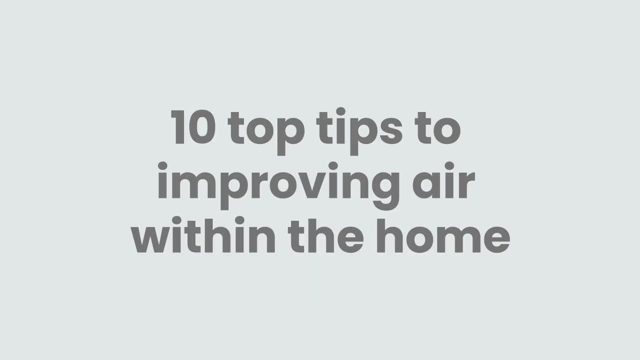 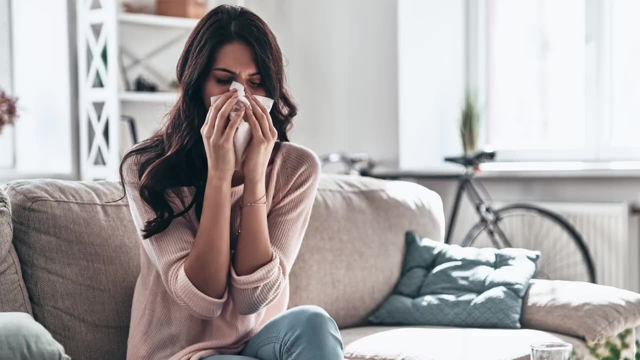 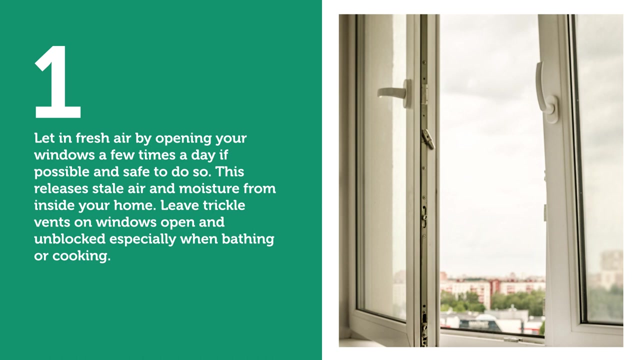 Here are 10 top tips to improving air within the home. Our top 10 tips to better indoor air quality: 1. Let in fresh air by opening your windows a few times a day if it is possible at home. Let in fresh air by opening your windows a few times a day if it is possible at home. 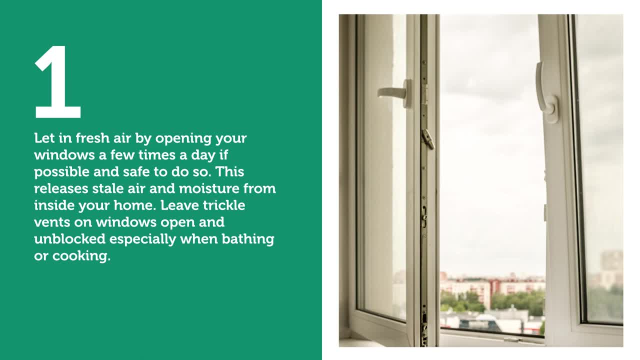 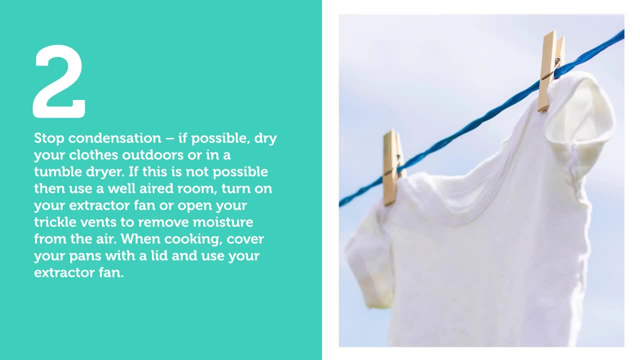 This releases stale air and moisture from inside your home. Leave trickle vents on windows open and unblocked, especially when bathing or cooking. Leave trickle vents on windows open and unblocked, especially when bathing or cooking. 2. Stop condensation. If possible, dry your clothes outdoors or in a tumble dryer. 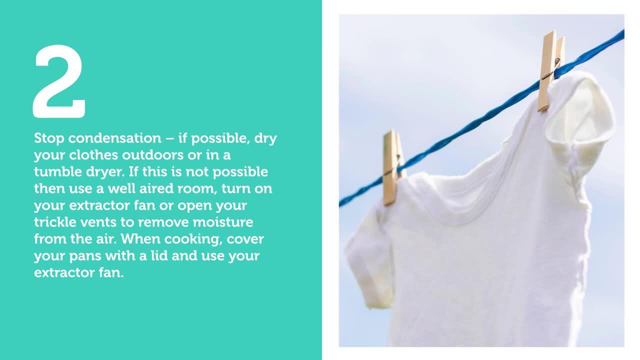 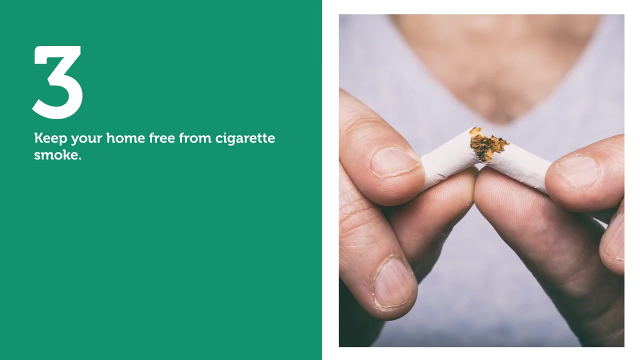 If this is not possible, then use a well- aired room. turn on your extractor fan or open your trickle vents to remove moisture from the air when cooking, cover your pans with a lid and use your extractor fan. three, keep your home free from cigarette smoke for keep warm by making sure your house is. 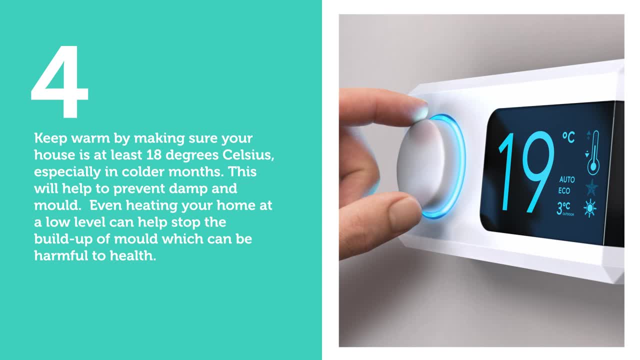 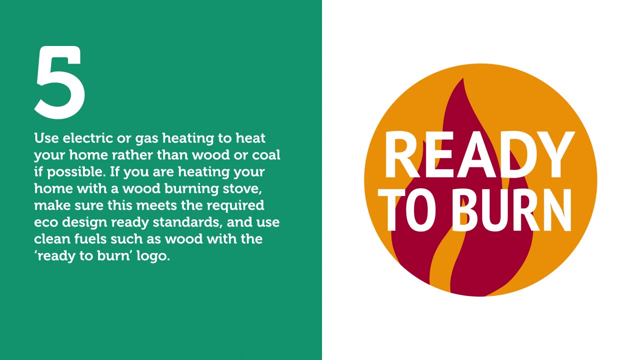 at least 18 degrees Celsius. especially in colder months. this will help to prevent damp and mold. even heating your home at a low level can help stop the buildup of mold, which can be harmful to health. five: use electric or gas heating to heat your home rather than wood or coal, if possible. if you are heating your 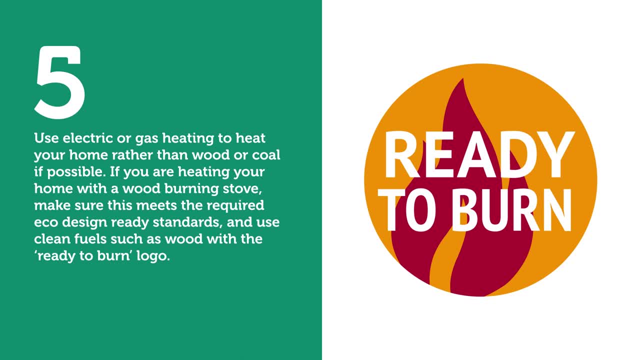 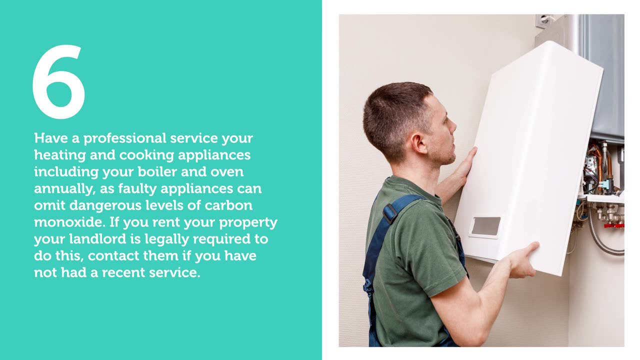 home with a wood-burning stove, make sure this meets the required eco design ready standards and use clean fuels such as the wood with ready to burn logo six. have a professional service your heating and cooking appliances, including your boiler and your oven, annually, as faulty appliances can emit dangerous levels of. 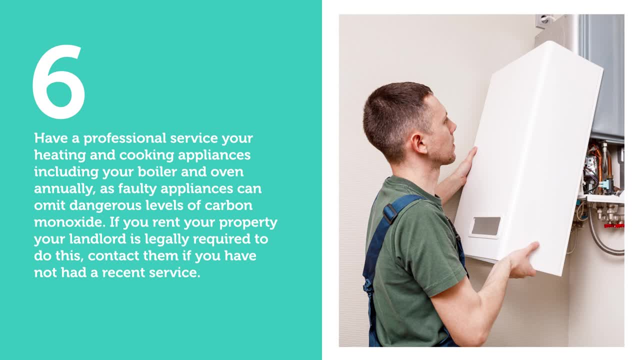 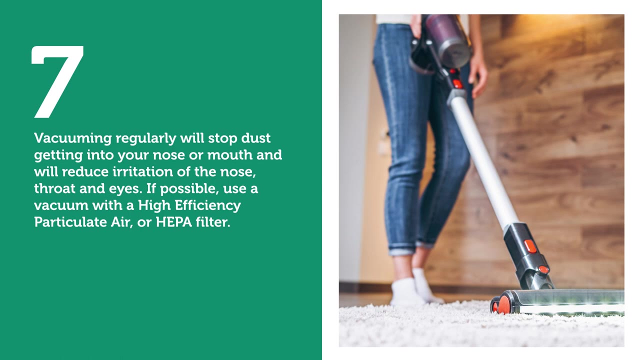 carbon monoxide. if you rent your property, your land lord is legally required to do this. contact them if you have not had a recent service. seven: vacuuming regularly will stop dust getting into your nose or mouth and will reduce irritation of the nose, throat and eyes. if possible, use a 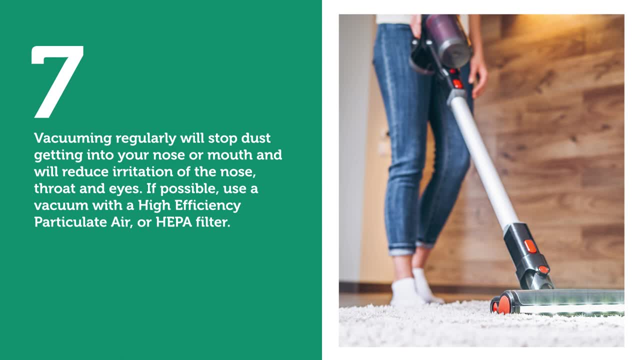 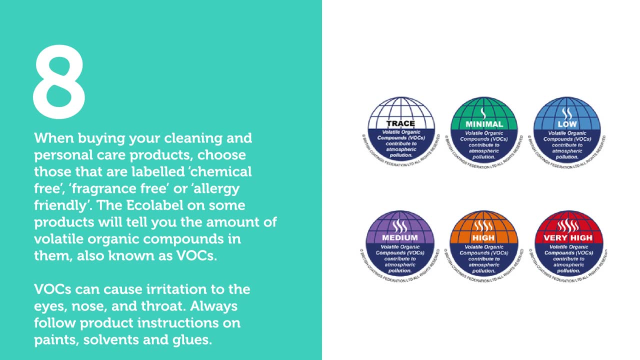 vacuum with a high efficiency particulate air or HEPA filter. eight: when buying your cleaning and personal care products, choose those that are labeled chemical free orHuh the money it comes. fragrance free or allergy friendly- The eco label on some products will tell you the amount. 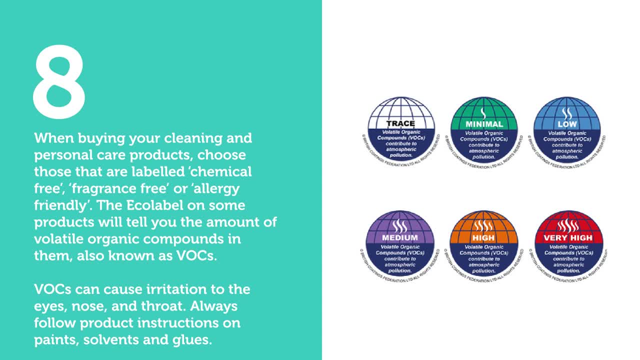 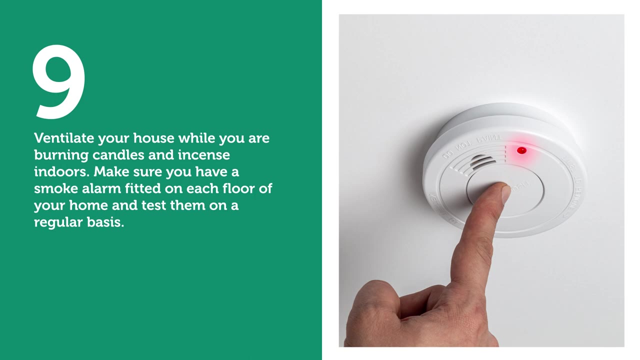 of volatile organic compounds in them, also known as VOCs. VOCs can cause irritation to the eyes, nose and throat. Always follow the product instructions on paints, solvents and glues. 9. Ventilate your house. whilst you are burning candles and incense indoors, Make sure you 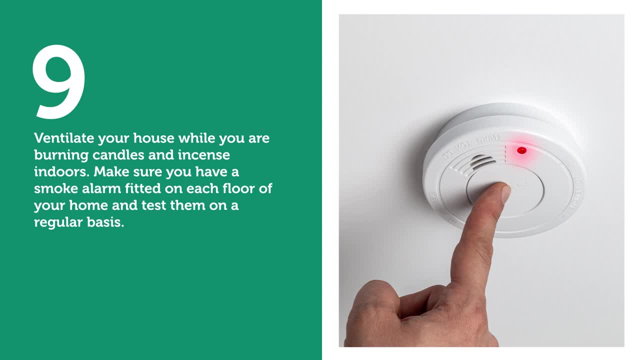 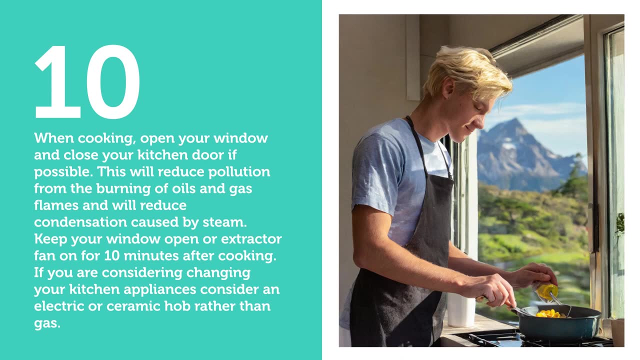 have a smoke alarm fitted on each floor of your home and test them on a regular basis. 10. When cooking, open your windows and close your kitchen door if possible. This will reduce pollution from the burning of oils and gas flames and will reduce condensation caused. 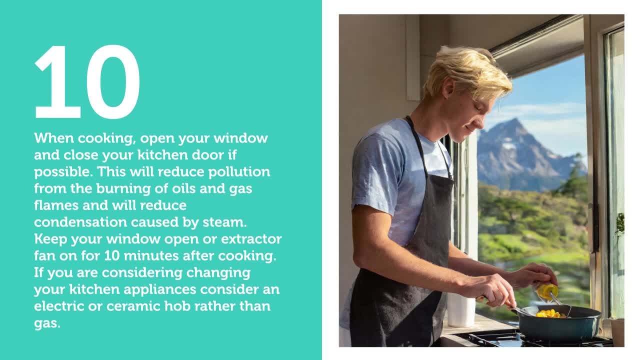 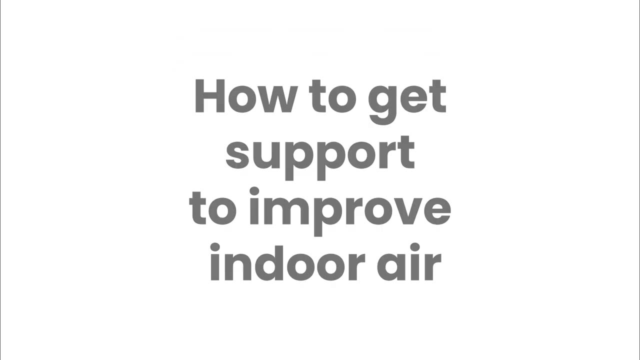 by steam. Keep your window open or extractor fan on for 10 minutes after cooking. If you are considering changing your kitchen appliances, consider an electric or ceramic hob. 11. How to get support to improve indoor air. What we do indoors. how we cook clean. 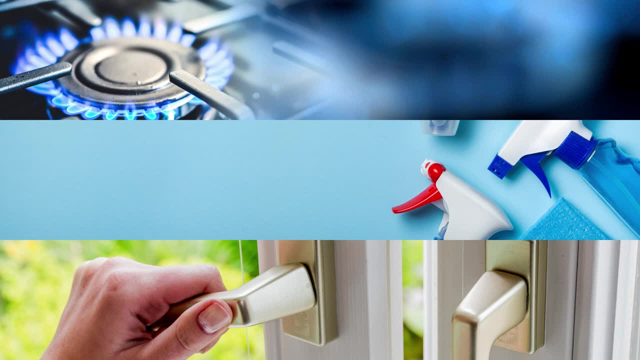 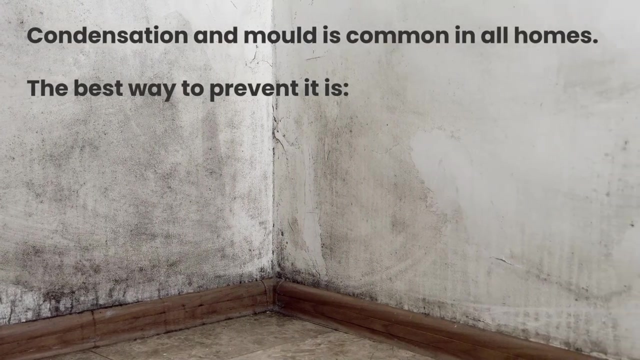 and ventilate can provide us with a safer and more comfortable home environment. However, sometimes help may be needed to improve our living conditions, to improve our health and well-being. 12. Dampen mould, Condensation and mould is common in all homes. The best way to do this: 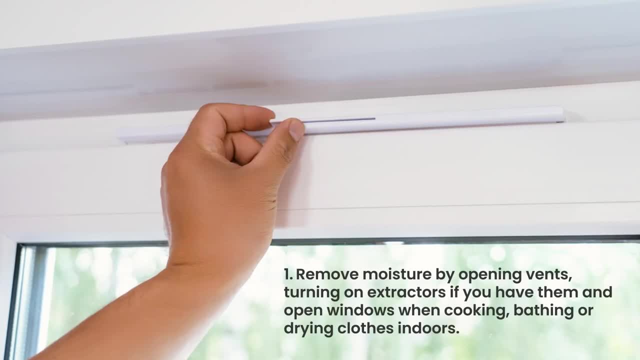 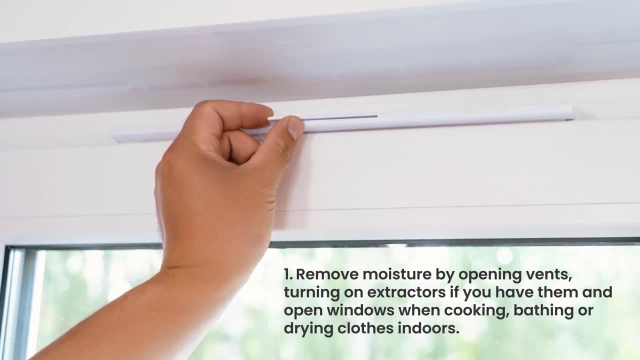 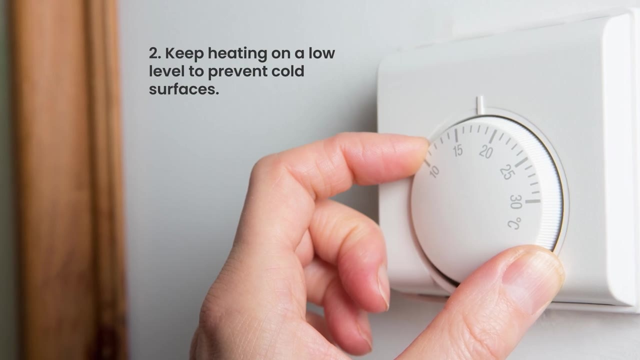 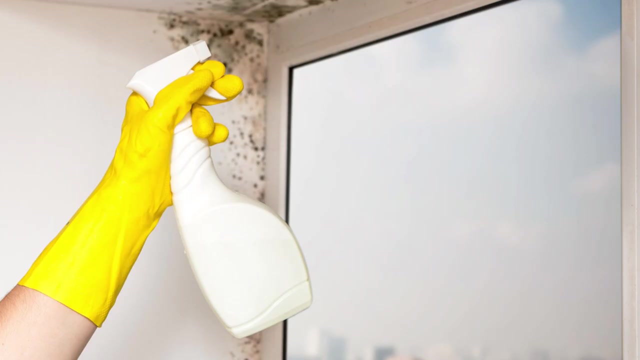 to prevent this is: 1. Remove moisture by opening vents, turning on extractors, if you have them, and opening windows when cooking, bathing or drying clothes indoors. 2. Keep heating on at a low level to prevent cold surfaces. 3. Wipe down condensation that forms on windows, walls and tiles. 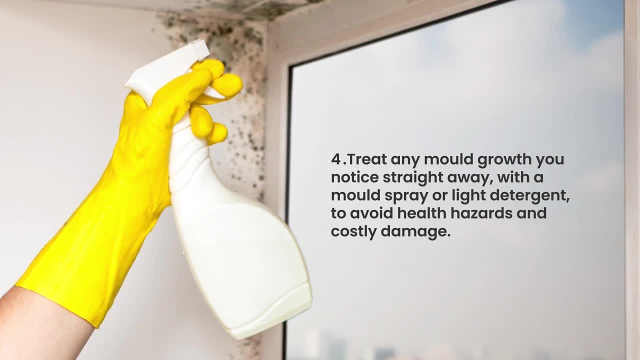 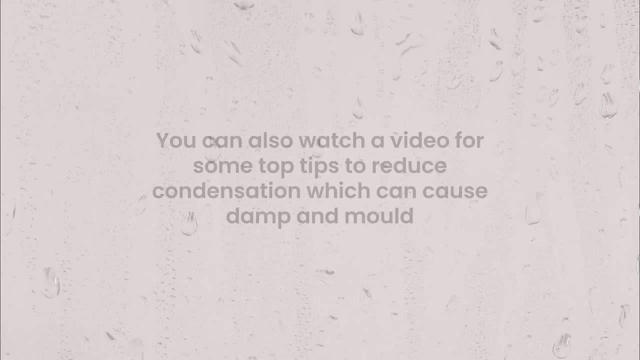 4. Treat any mould growth you notice straight away with a mould sprayer. 5. Use a sprayer to remove moisture from your windows and windows. 6. Use a sprayer to remove moisture from your windows and windows. 7. Use a sprayer or a light detergent to avoid health hazards and costly damage. 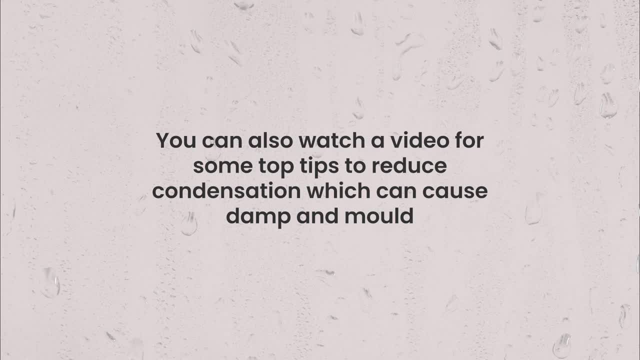 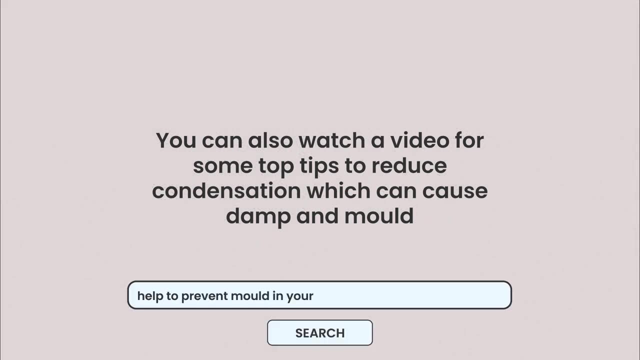 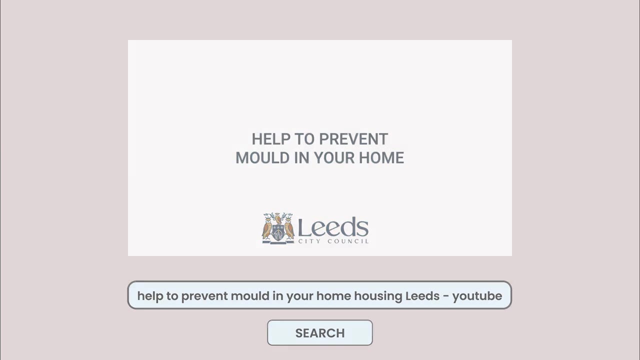 You can also watch a video for some top tips to reduce condensation which can cause dampen mould. Search for Help to prevent mould in your home housing leads dash YouTube in your internet search engine If the damp problem gets worse or you aren't able to deal with dampen mould growth by yourself. 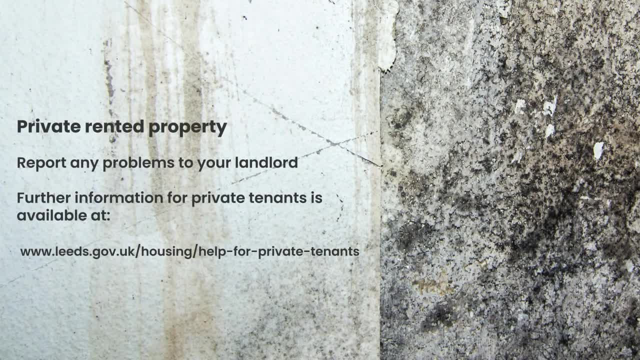 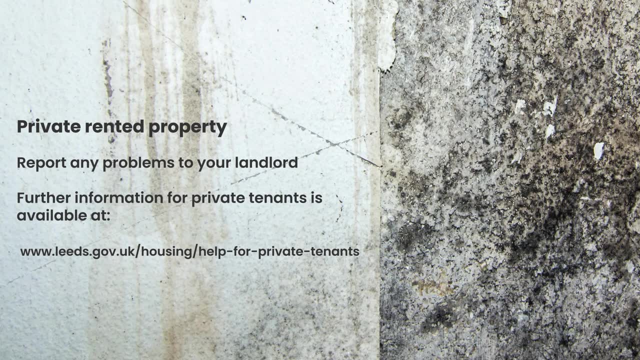 then please tell your landlord. If you live in a private rented property, you should report any problems to your landlord, who will be able to take any action needed. Further information for private tenants is available at wwwleedsgovuk- wwwleedsgovuk. 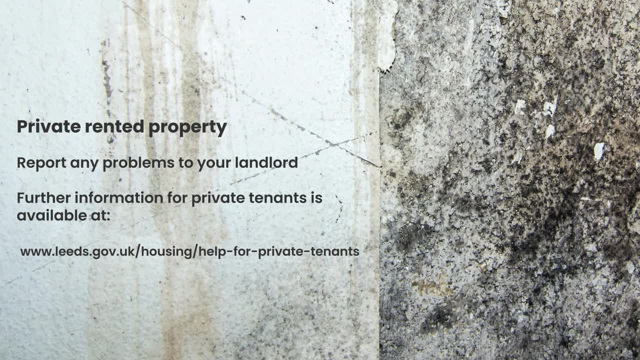 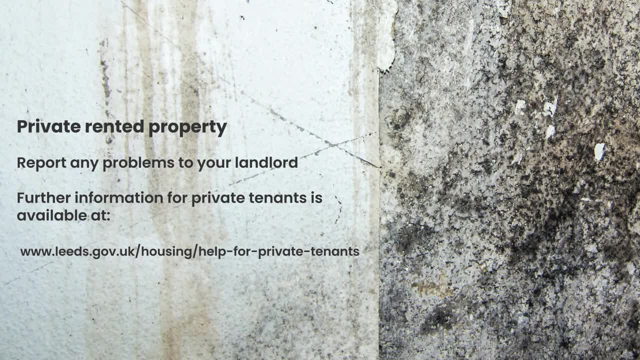 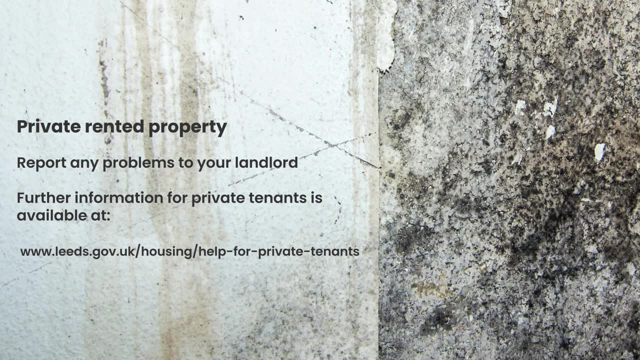 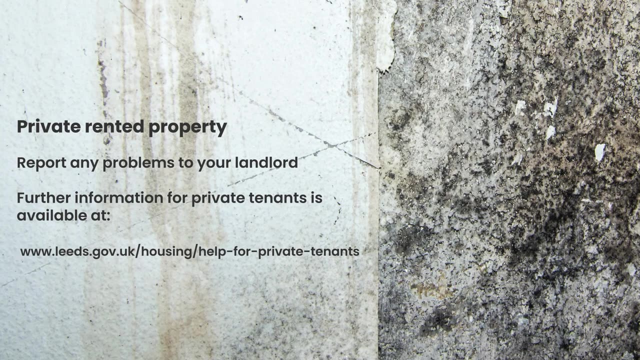 wwwleedsgovuk, wwwleedsgovuk, wwwleedsgovuk, wwwleedsgovuk. The council may be able to help if the problem is caused by your landlord not making repairs that are causing or making any dampen mould worse. 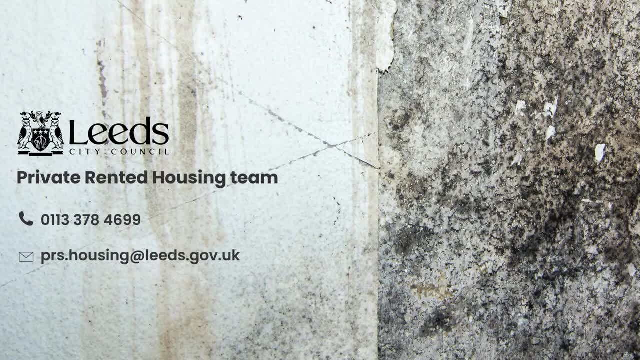 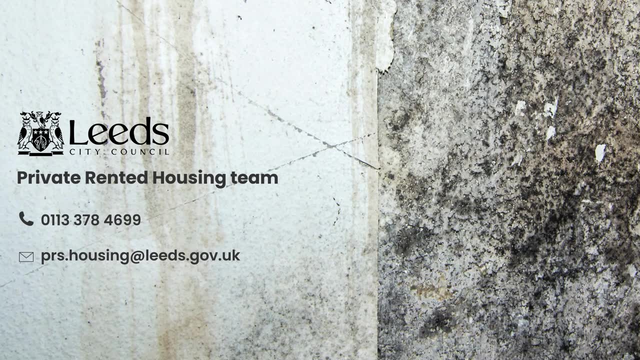 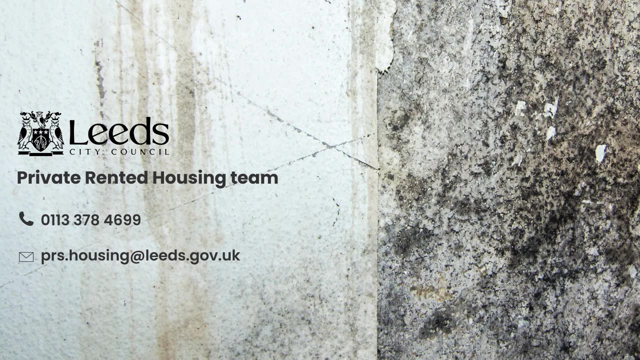 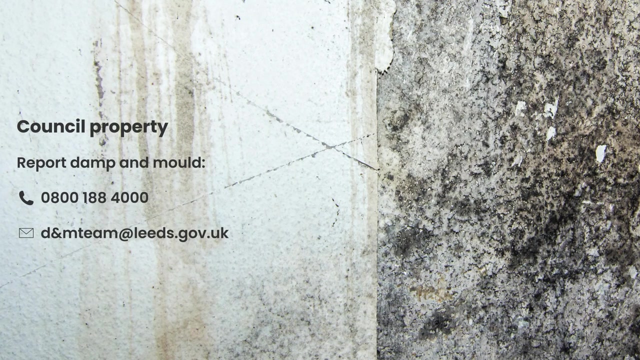 You can contact the Private Rented Housing team on 0113 378 4699 or email prshousing at leedsgovuk. If you live in a council property, you can report dampen mould by calling 0800 188 4000.. 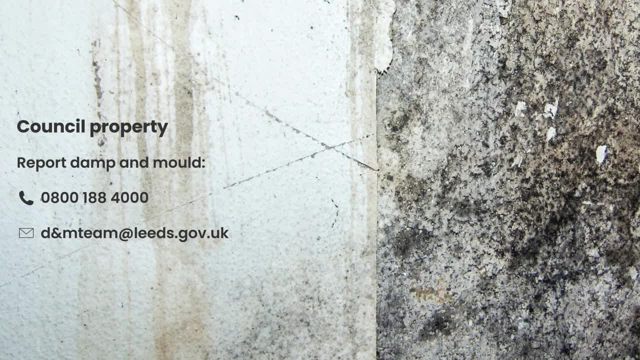 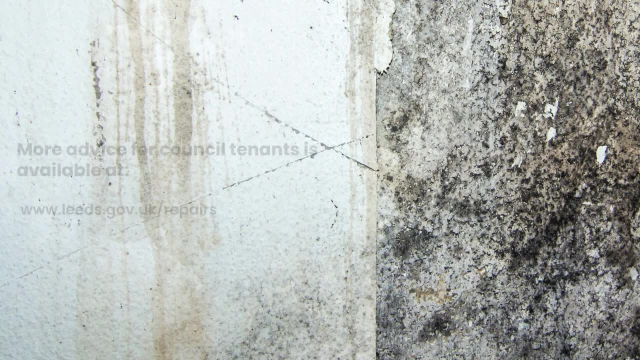 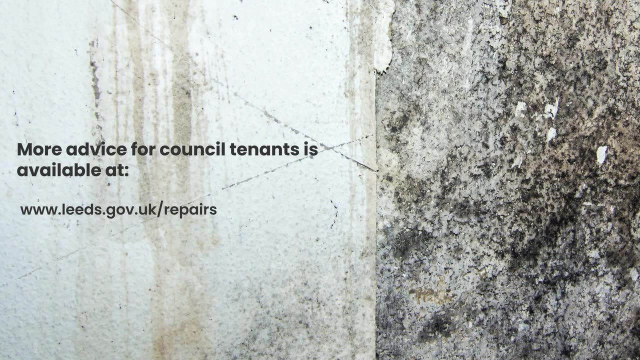 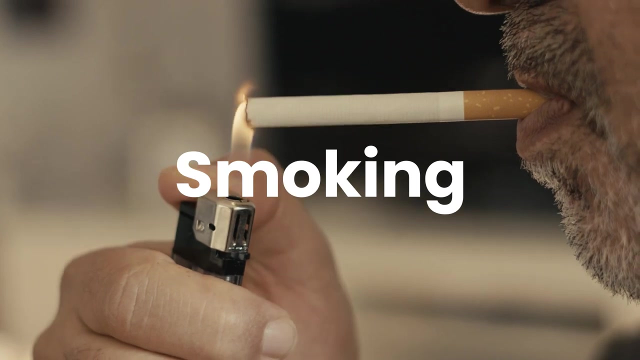 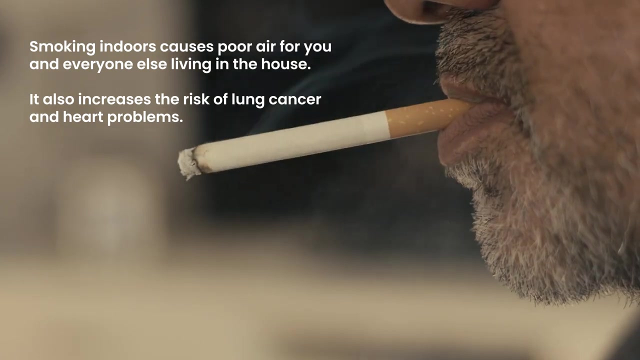 Or by emailing d&mteam at leedsgovuk. More advice for council tenants is available at wwwleedsgovuk-repairs. Smoking- Smoking indoor causes poor air for you and everyone else living in the house. It also increases the risk of lung cancer and heart problems. 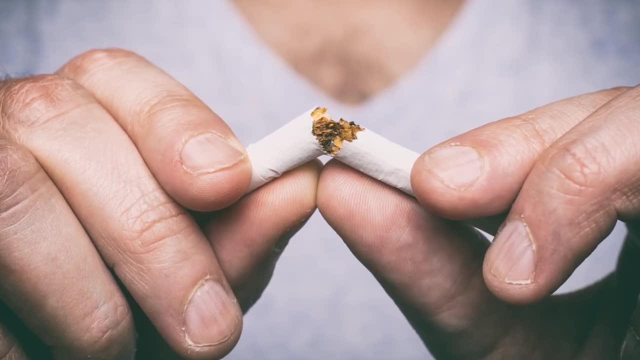 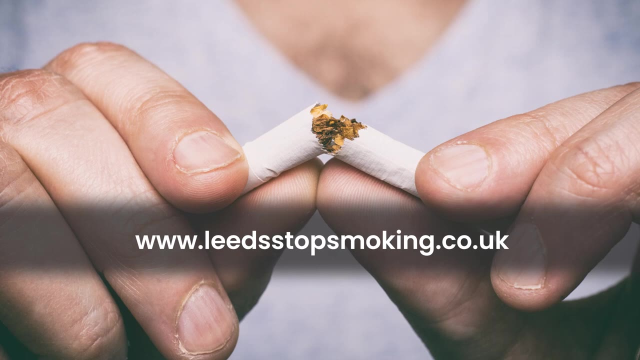 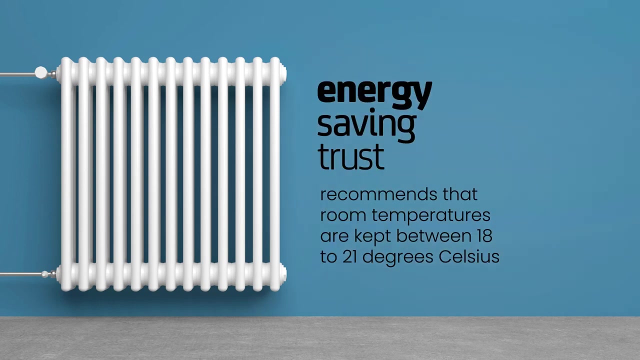 Quitting smoking has several health benefits. To find out more and to receive support to stop smoking, visit wwwleedsstopsmokingcouk. Keeping warm: The Energy Saving Trust recommends that room temperatures are kept between 18 to 21 degrees Celsius to prevent heatstroke. 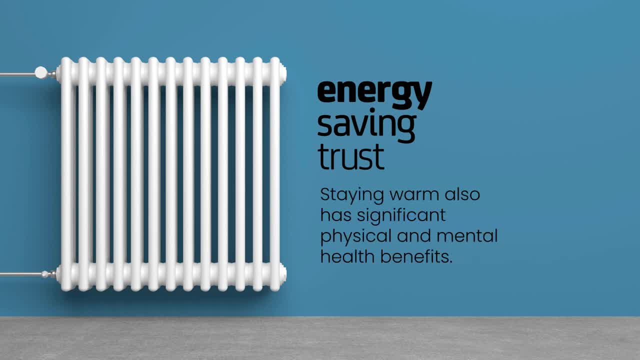 Staying warm also has significant physical and mental health benefits. For help and advice on organisations offering affordable warmth grants, visit wwwleedsgovuk. forward slash housing. forward slash. make dash your dash home. dash more dash energy, dash efficiency. wwwleedsgovuk forward slash housing forward. slash. make dash your dash home. dash more dash energy, dash efficiency. 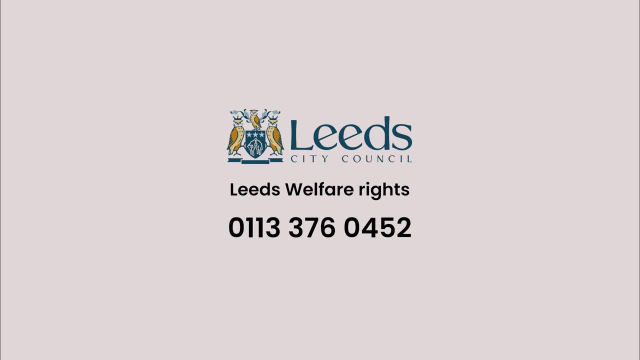 Leeds Welfare Rights will also be able to make sure that all appropriate benefits are being claimed and signpost you to any other services they feel are able to support you. If you would like to contact Welfare Rights, call them on 0113 376 0452..